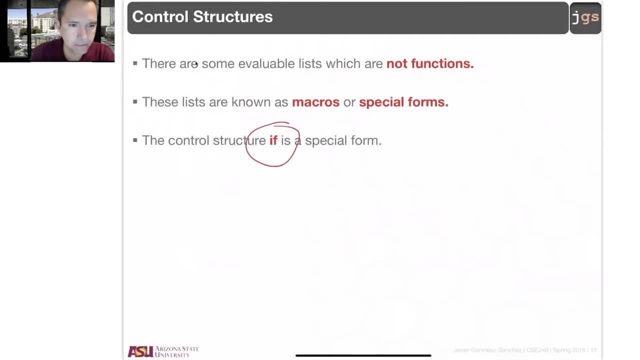 already know the if condition Theoretical background. The control structures in Lisp are not considered functions, even though they look like functions and I am going to show you. but officially they are macros, not functions. Let me show you an example. 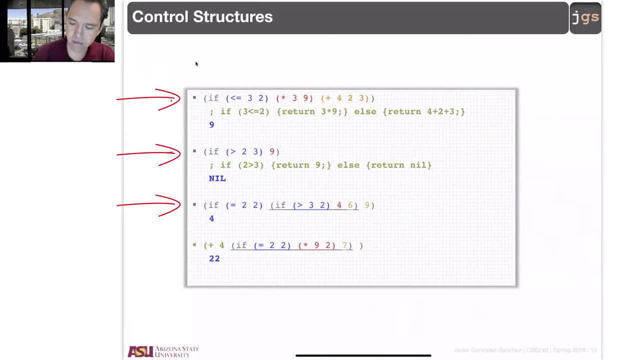 These ones, Each of these, an if-else condition. What is the black, the blue, the red and the orange part? You can figure it out and I use the colors to facilitate this Number one if you want to create an if-else condition, as usual. open parenthesis. closing parenthesis. As usual. 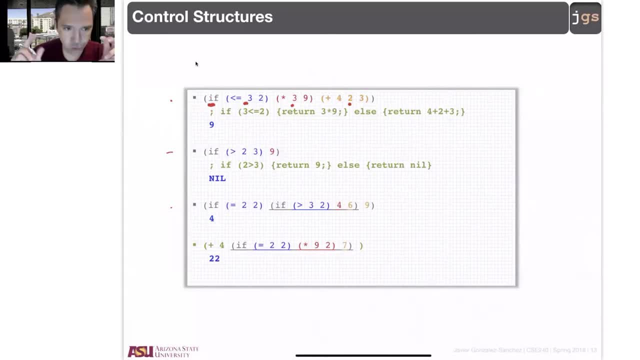 the first element after the open parenthesis, the name of the function, in this case the macro if, And you can use if, uppercase, lowercase or a combination- For this language it's not going to be any difference- So if. 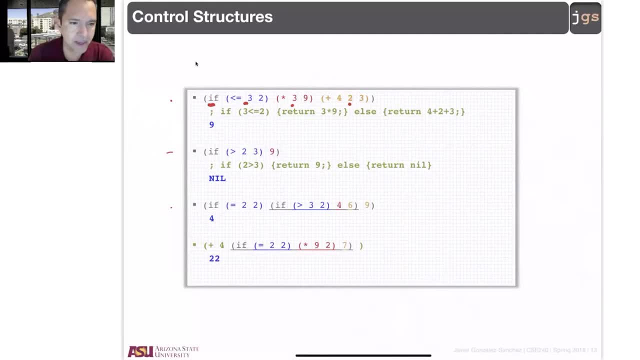 And then the first element. The first parameter is a predicate. The first parameter is something that returns true or false, In this case in blue. true or false. The three is lower or equal to two. If the result is true, this statement, the second parameter, is going to be executed. If the 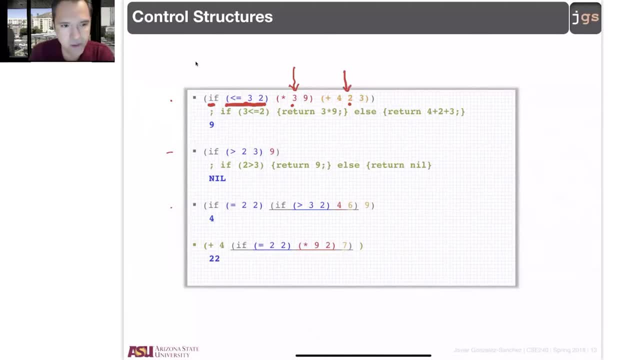 result is false, the orange one is the one that is going to be executed. The equivalent to that one is my comment here in green. Remember, semicolon is the beginning of a comment and you can start a comment in a new line or at the end of the previous line. 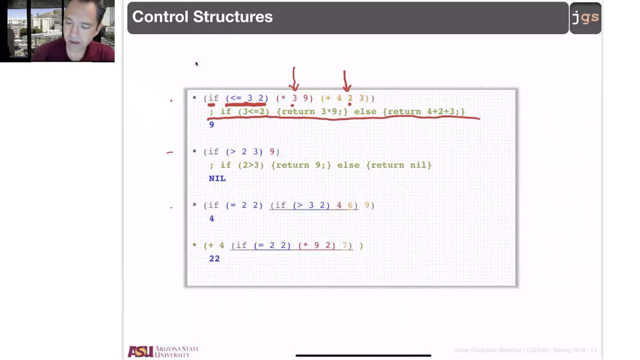 What can I do if I do not want to have the else part, If I do not want the else, I want nothing to happen. if the condition is false, The only thing that I need to do is do not provide the second parameter. So, 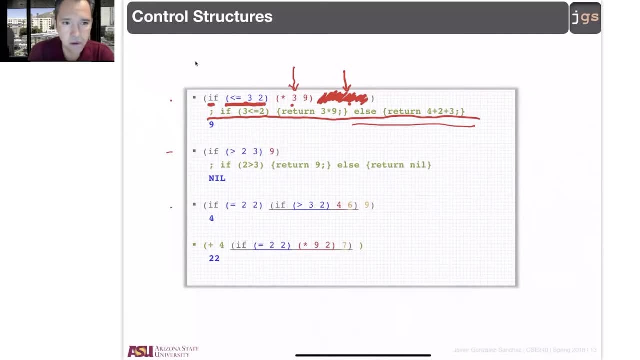 for the macro. you have two options: Option number one: two parameters. option number two: three parameters. If you use two parameters or three parameters, always, always, always, the first one is the condition. the two next parameters are going to be the instructions. 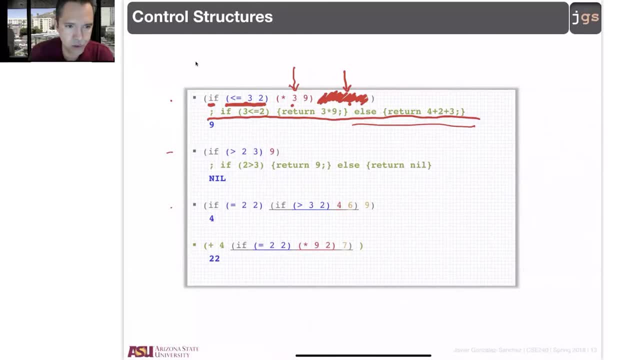 for they if and the instructions for the else, The instructions to be executed when the condition is true. on instructions we executed when the conditions for that shit. Even though the condition- the if- is a macro, the behavior is going to be the same as the behavior of a function. Any function returns. 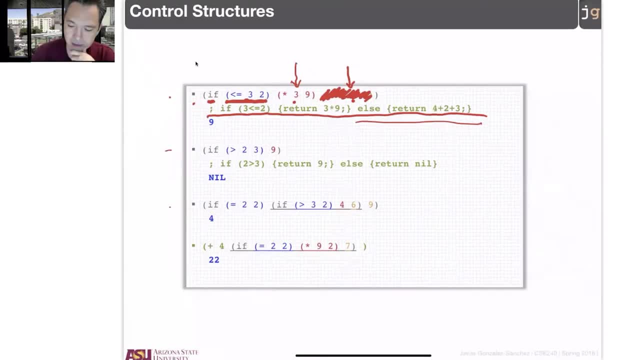 a result, In this case this number. and you can be wondering why. Well, that is the value that is being returned by. whatever is the result of the instruction that is executed In this case, if I check the condition, it's going to say false. It's going to execute the else part. 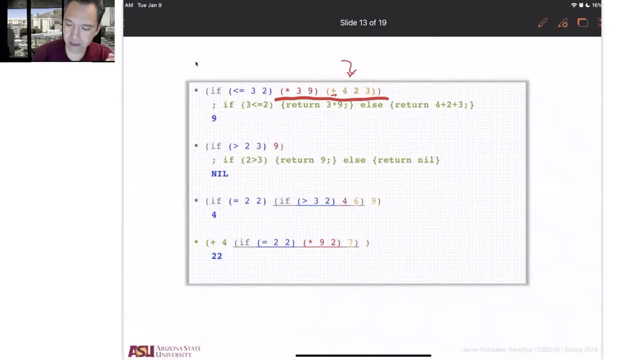 This addition is going to be executed. The result of the addition is the result for this instruction and also is going to be the result for the complete if else condition And the equivalent of this in C, C++, should include this return. So example one. Example two: Because the if else returns something is fine to use a single value. 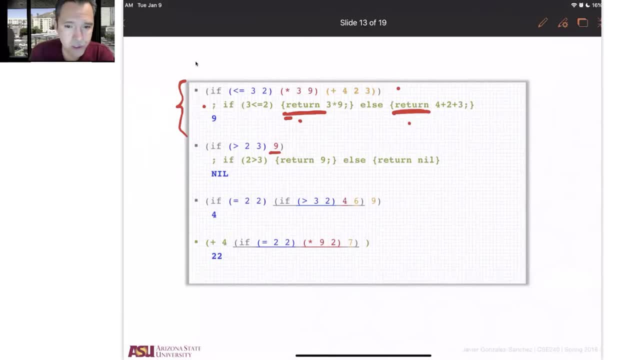 there. So in this case, this is a condition. It's asking if the two is greater than the three. If the condition is true, this is going to be the value that is going to be returned. In this case, we are not providing an else. 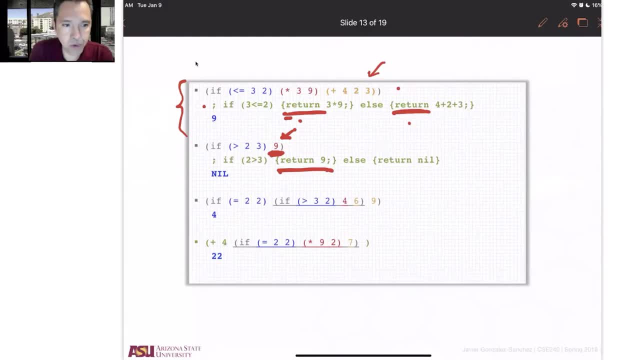 Like we did before, if you do not put an else to an if else condition and the condition here is false, the result for the full instruction is going to be nil. Remember that we use nil in Lisp for false, but also nil is our equivalent to empty. So in this case, if the condition were true, I return an else. 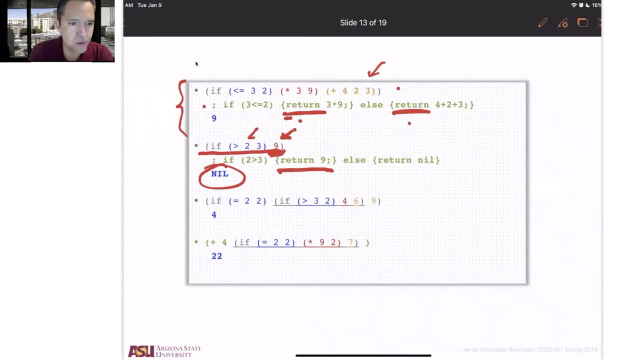 My condition is false. Therefore, it's going to return nil. In the next one, you can put an if and have other ifs inside. What if I ask you to translate this one to Java, C, C++? I have an if, this one, that is the one that is outside. 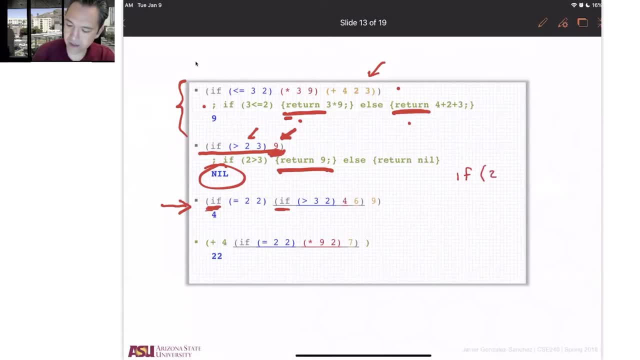 The condition for that one is this: to give the value to this condition. The condition for that one is this: to give the value to this condition is this: two equal, equal two. very, very important. remember that the equal equal, the comparison in lisp- is only one equal. so this is not a signature. so if two equal, equal, two is this part. 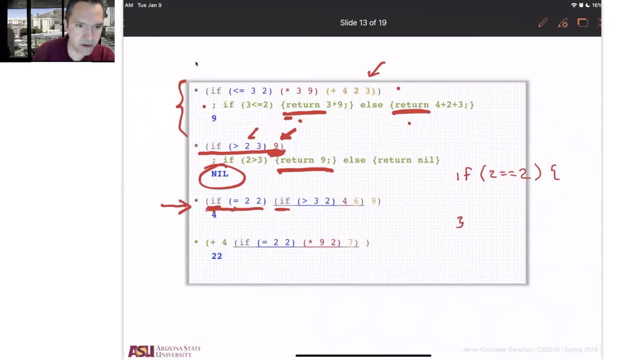 and i need something in the if part and maybe i have an s part. now, if i review here, i have one parameter that is going to be: from this open parentheses and move on till this closing parentheses. again, i put colors to try to facilitate the lecture, so you know that the 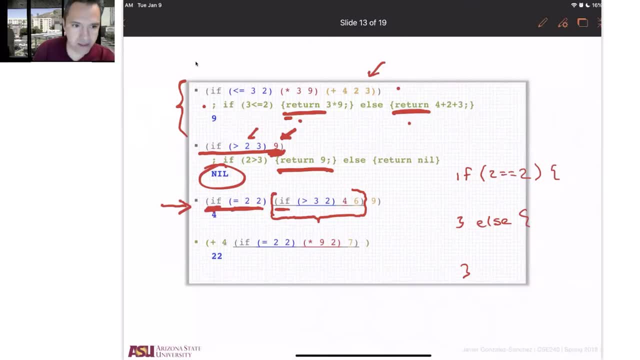 parentheses in blue is one thing, and then something in red, something in yellow and the gray black parentheses is the one that is closing the if that is inside. so this one is one part and this nine is the second parameter for the first if. so that nine is kind of the else part. the first part is this one. that is an other if condition that is inside. 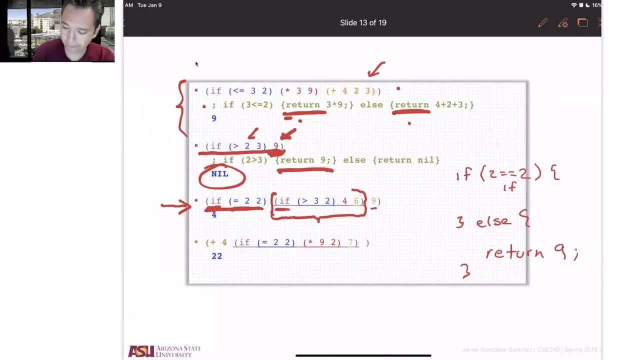 of the first one inside of the true part. for the third one. we have another condition here: you can put the else part inside of the first one, you return four, and inside of the else part you return six. so you have these two. if else, here you can start noticing the problem with the parentheses. 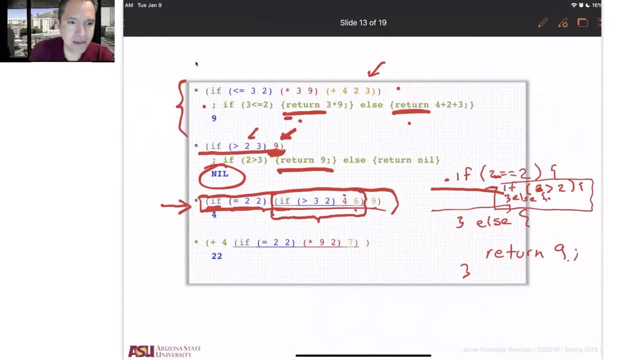 good thing about the parentheses is a very, very, very simple syntactical rule. so this idea of everything is: open parentheses, closing parentheses. the instruction on the parameters is simple but- and in some point it's kind of complex, if i remember, of the colors to figure out which parentheses is related with which one. 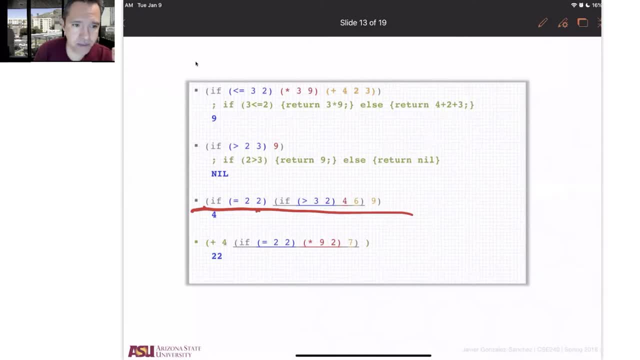 so a second thing for the if condition. in lisp you can use an if condition like this one as a parameter for another function because, remember, the if return a value, so you can put the if inside of the call to a function and basically the value that that if 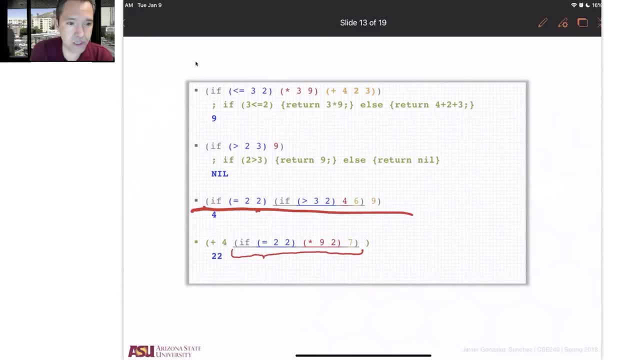 condition returns is the one that the function is going to be using. So in this case, for instance, I have this instruction plus four and I am going to do the addition of four plus something and that something is going to be whatever result in. 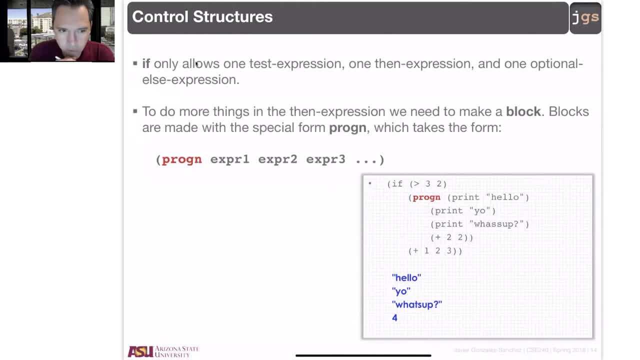 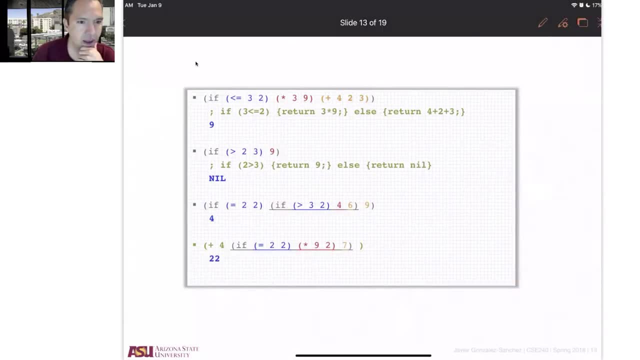 this condition. Now there is one problem. So far, the examples that I show you are like the if the condition and only one line inside. Even with the else, only one line inside. What if we want to have an if-else condition with multiple lines? 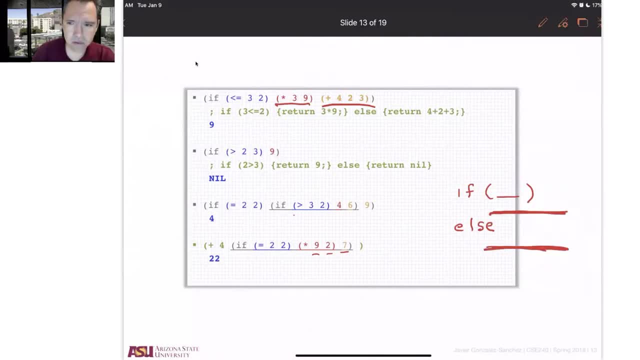 Well, you know, in Java, C, C++, if you need more than one line, You add the curly brackets. But remember, you only need the curly brackets when you want to put together multiple lines. Now what happens here? if I want to put together multiple lines? 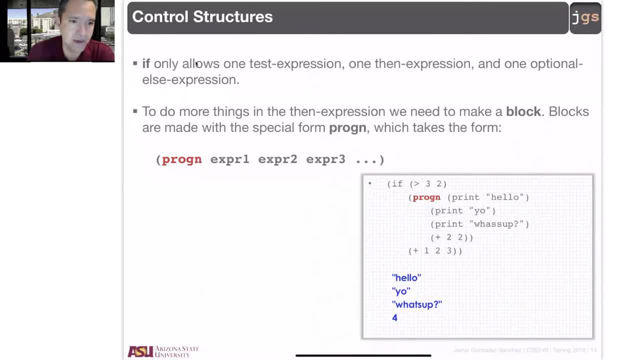 I cannot use the curly brackets. The curly brackets do not exist in Lisp, So instead of using the curly brackets to create this block, what I am doing is I am going to use is another function With this name: procn. the use of this. 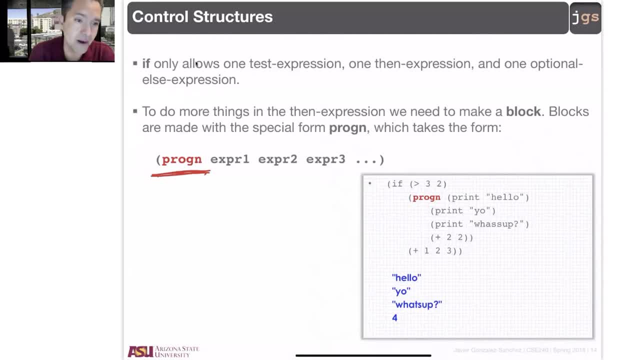 function is to put together several lines. You can think about this guy like your equivalent for the open curly bracket and therefore closing curly brackets. Every single time that you need something like this, you are going to use this guy. So one example: I have an if condition here. Notice that this open 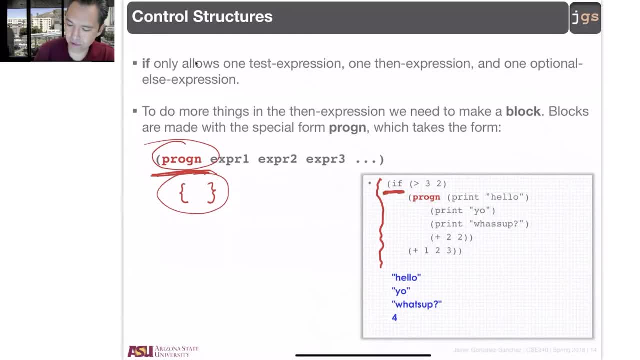 parenthesis is going to close here. All this is my. if The condition is the first parameter, the second element after the open parenthesis, The next thing is the instruction that I want to execute when the condition is true. But I want to have multiple instructions, So what I do is: 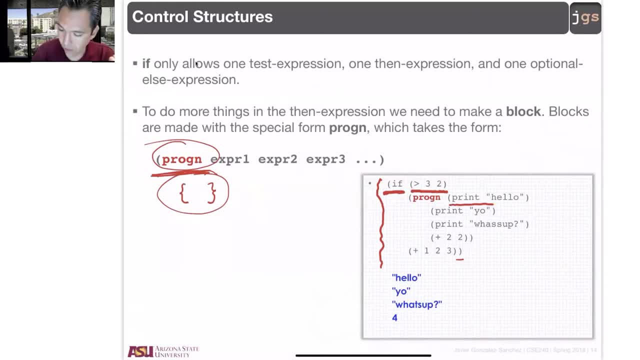 put those instructions one, two, three, four instructions that I want to execute when the condition is true, all my instructions together inside of another one. Notice this parenthesis. So I put a name for a function, this name and that. 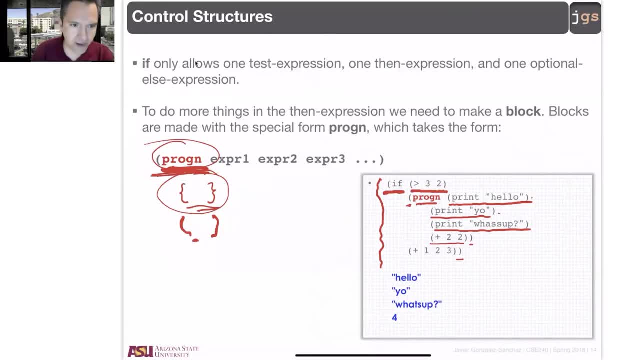 is the name for the function. that replaces the name for the function. Now replace the curly bracket. So now, all of these together are the instructions that I want to run when the condition is true. And then this one is the instruction that I want. 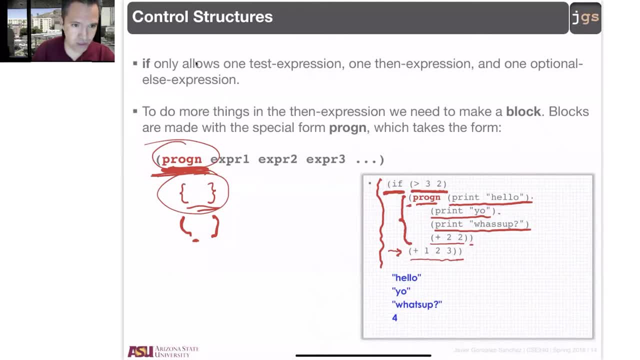 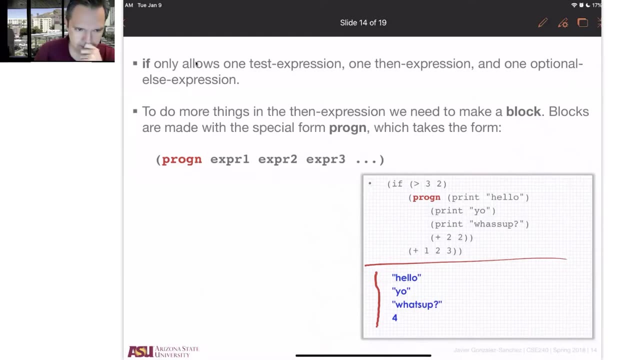 to run when the condition is false. So PROC end to create block of instructions. But for this example. what is the output of this example Number one? if we execute the program it's like the condition is true or false. Three greater than two right True. 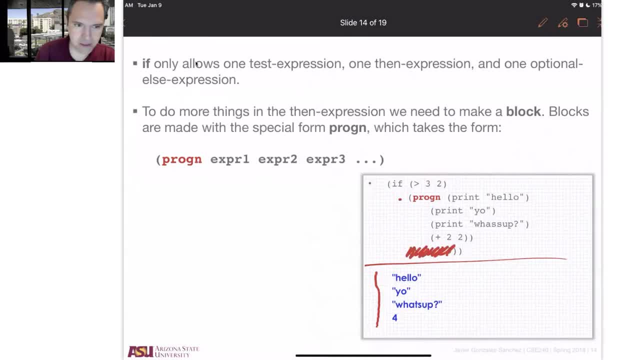 So this instruction is not going to be executed- never, because this one is the else part. The program is going to run whatever is inside of my PROC end block First one. this instruction is going to be executed. I am going to have a hello. That hello is because the print 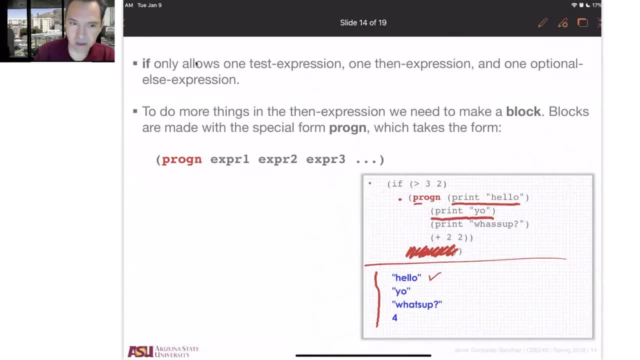 instruction: This instruction is going to be executed. I have this word here because this print, This instruction is going to be executed. I am going to have this one because that print instruction. Finally, this one. This one is not printing, But this one is. 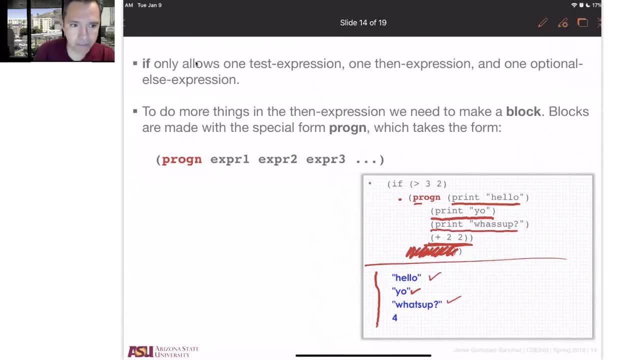 going to be executed. This plus is a function When I run the program. I am going to solve also a four because of this, This if condition returns something. Well, when you have only one line, like in the previous examples, it's obvious that the if returns the value of that. 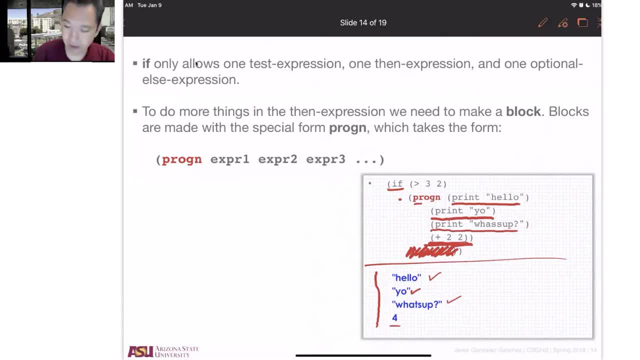 line. What happens when you have multiple lines? What happens when you have something like this? Well, the easy solution: You return the value of the last line that you execute. So in this case, the last line is this plus two, two. This function returns a value, the four. That value is the same. 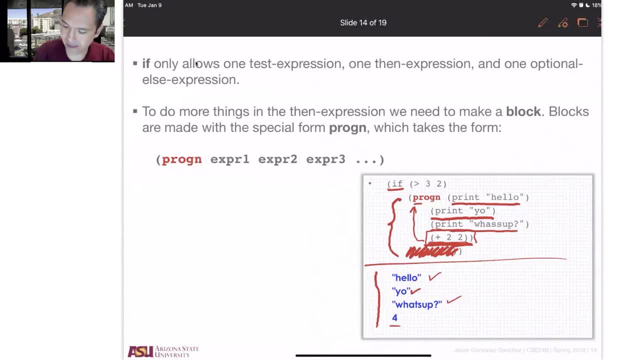 value that is going to be returned by this function, PROC end, And that one is the same value that is going to be returned by the if function And that is the value that you are going to show on the screen at the end. What happens? 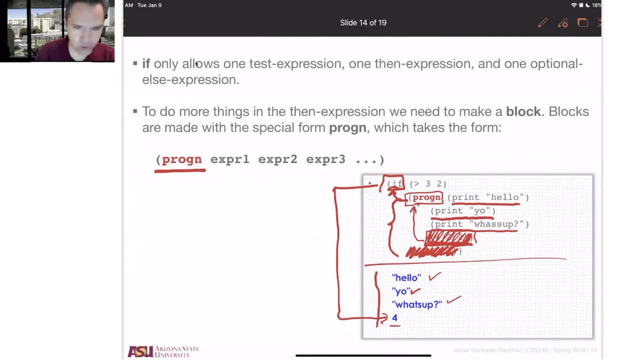 if I remove this plus right, It's going to return whatever print return. What is the return of a print? The same value that is printed. So if I remove this one, the last line is the print what's up, And therefore, what's up is the value returned to PROC end. 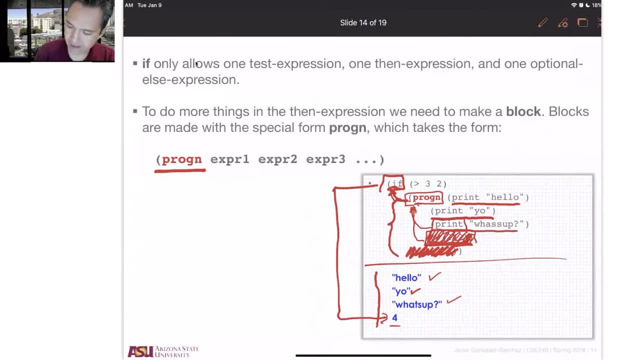 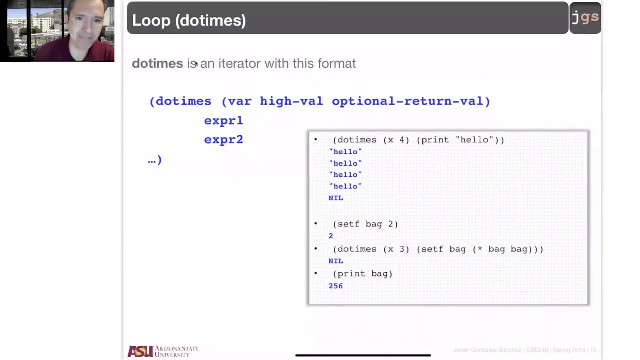 And it's the same value that PROC end returned to the if. And then, instead of this four here I will have this again: The loops. We have multiple options for loops in Java, CC++, In particular with Lisp. we're going to move forward with this option: The instruction, the function that is going to 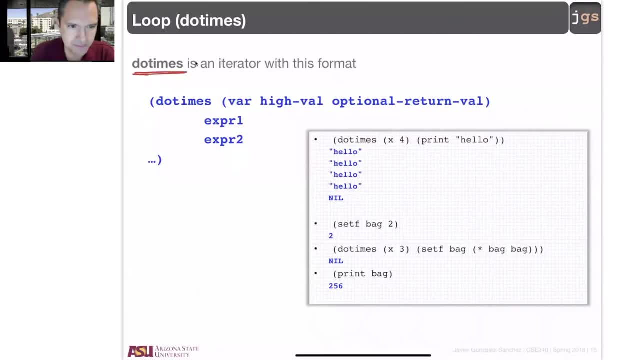 help us to do loops is do times. Do times, As usual, open parentheses and closing parentheses. So in this case, opening here, closing here, The first thing after the open parentheses, the name of the function: do times And then 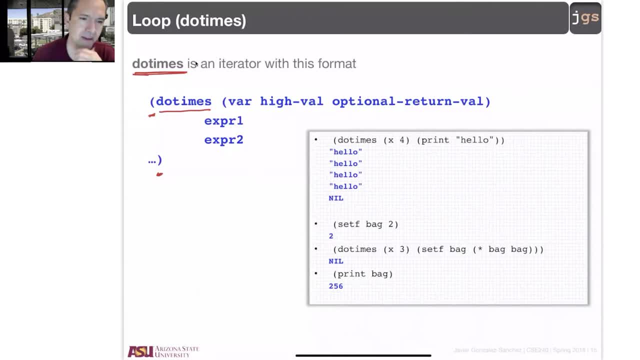 the parameters Parameters. This is the first time that the parameter for a particular function should be a list. So after do times, what you need to put is a list of elements which mean after do times. What you need to put after do times is a list of elements which 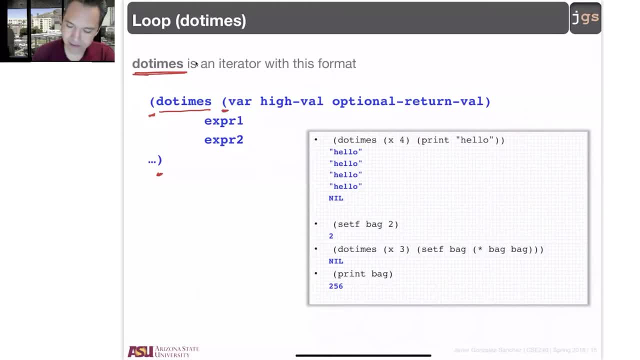 means after do times. what you need to put is a list of elements, which means after do times. you are going to open parentheses, and if you open the parentheses, well, you close the parentheses. after that one. everything else are the instructions that you want to execute. so you can have this instruction, this instruction or. 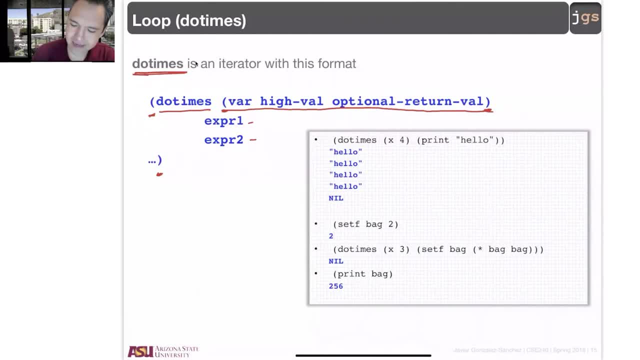 more now this list of parameters. the first element: for the first time, inside of a list, inside of parentheses, we are not going to put the name of a function, because that one is not a function in use, a list with values. the third one is the variable that we want to use, to be aware of in 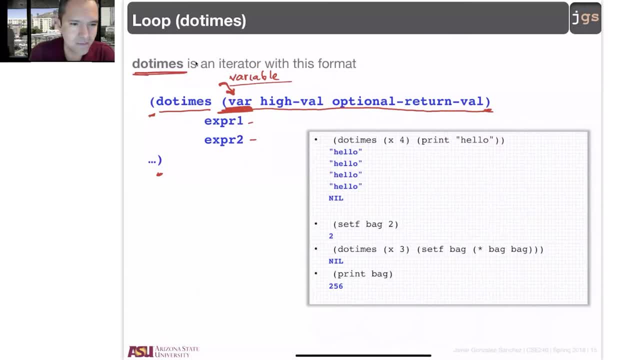 which of the following functions we are going to use to be aware of in which of the iteration we are. that one is kind of the. if you think about a for loop, this one is the equivalent to the variable that you put there, for the for loop is the variable that is going to help you to. 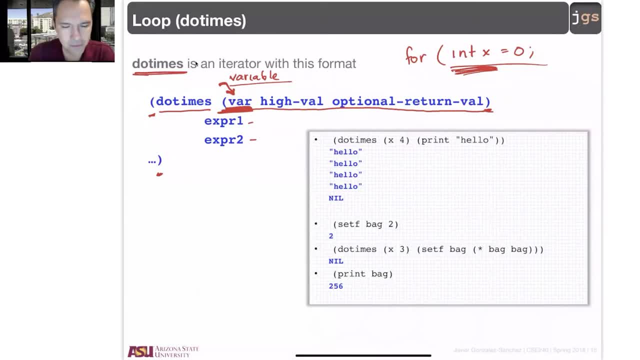 count how many times you have been inside of the loop. then inside of the same list, you have a value. a value of that represent how many times you want this loop to go. So in this case, below x and 4, I want the loop to run four times, so I put x. that is the variable. 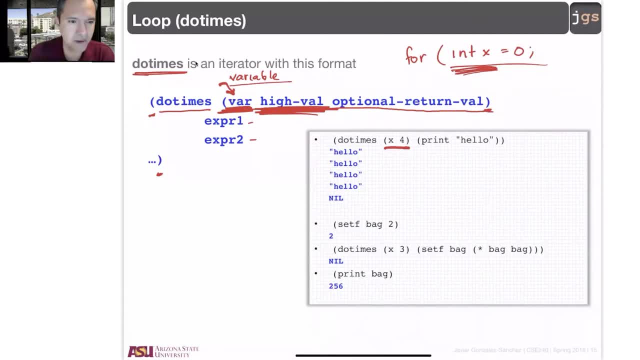 that I'm going to be using At some point. I can print x and I can print 1,, 2,, 3,, 4, or whatever, and I need to put the value- the value 4, because I want this loop to. 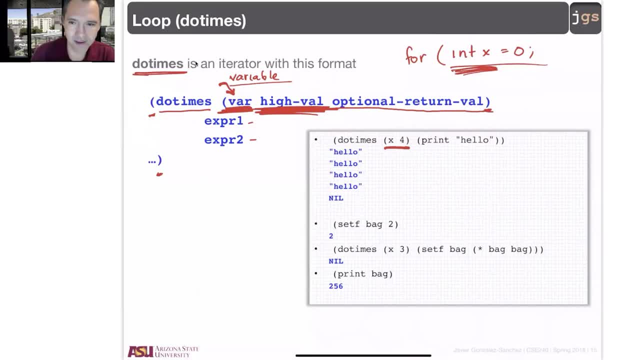 run four times Optional. I can put only two values, because that is what I need for the loop, or I can put three values. The third value is optional and if I put something here, that is the value that I want this function to return when the 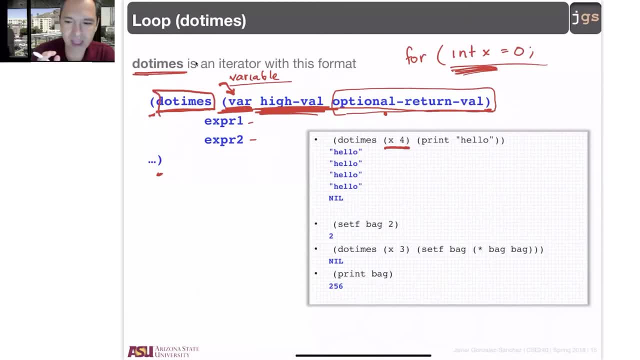 function finishes So that one is optional. The last one is my return value. In this case, we do not apply the rule that the return value is going to be the last one inside of the loop. The return value is whatever you put here, or if you do not put anything, like I did here, I just 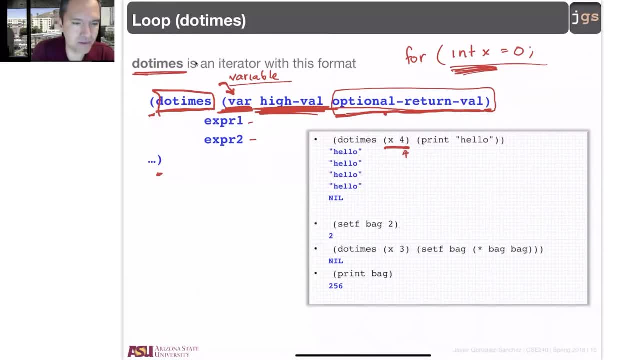 ignore the return value, my return value, the result of the doTime function is going to be something like nil Good. So doTime, the first part of the parameter should be a list, The first time that the list is not a function, And 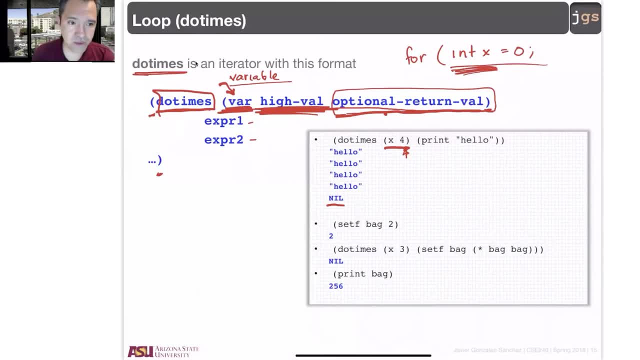 that list has at least two elements. The first one the name for a variable. The second one how many times I want the do to go. And optional, a third parameter that represents the value that I want to return, Anything that you want to return. 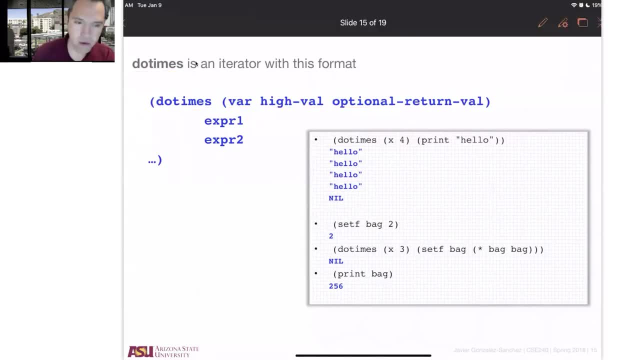 after this loop finishes. So reviewing the example: Parentheses- parentheses- DoTimes. And my variable is x And I want this one to run four times And the instructions that I want to run four times is this one: parentheses- parentheses. 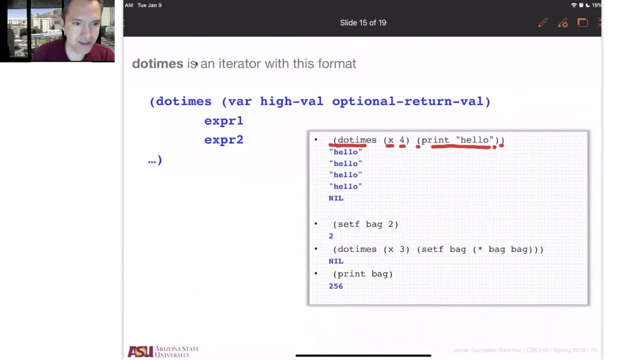 I want to print hello four times. The result: when I run the program, I have hello four times And because I do not specify any return value, the return value was nil. You are going to have as a return value the return value of the. 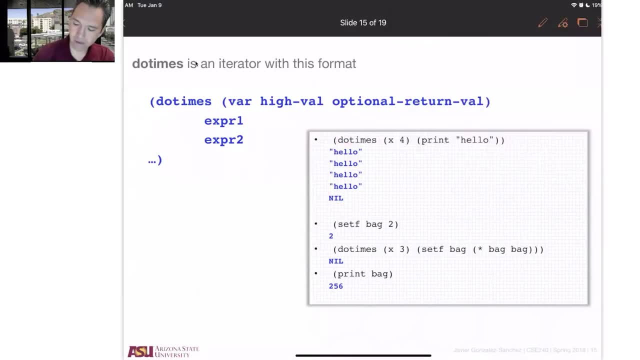 need The other example. We need variables Because you know if you want to do something inside of a for loop. sometimes I would like to have some kind of variable And inside of the for loop change the value of the variable. 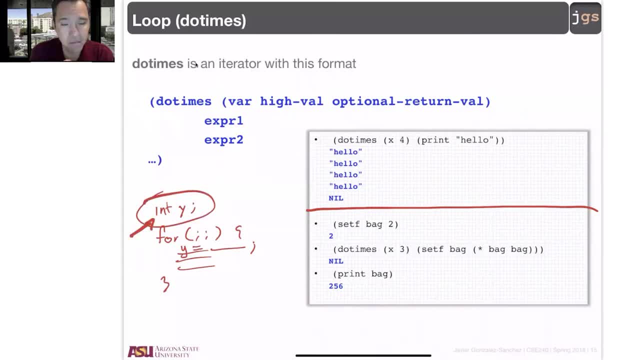 This is a good time to introduce variable declaration. The instruction that we're going to use to do something like this is this one. So if I want to create a variable int x and I want to put x, the value of five, the key of that line, 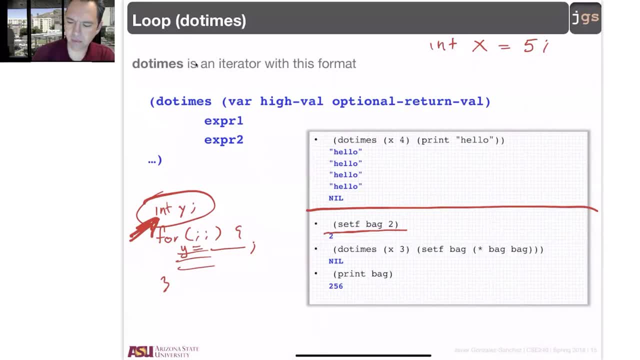 int list is open parentheses, closing parentheses. And then if I want to set the variable and the five, and let's use the word set and why not set f, the function set To create a variable in list, what you need is to provide a name. 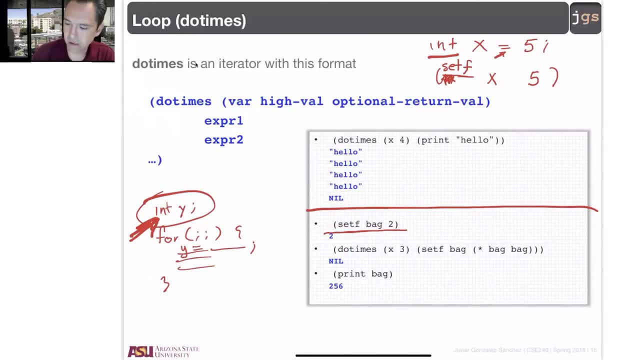 and provide an initial value. So the name and the initial value. In this case, I have this variable back. I put a number two inside. This is a function. The value that is going to be returning is going to be the value that's put inside of the. 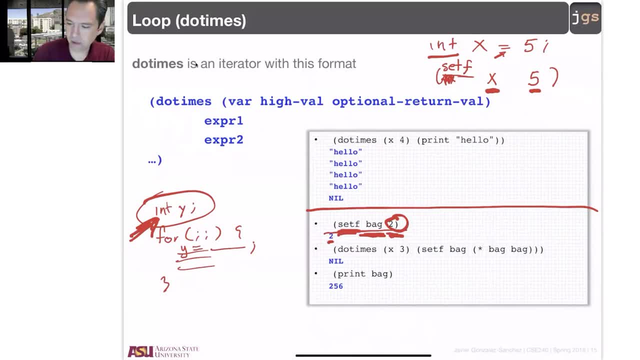 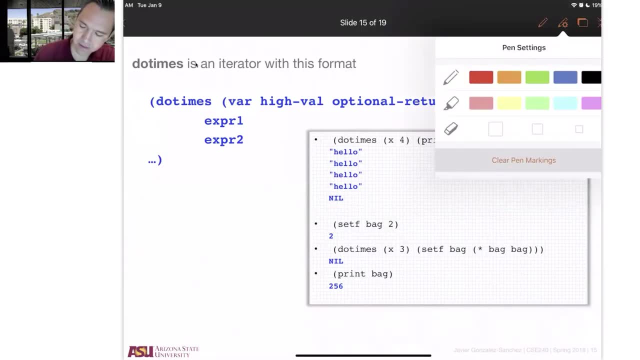 variable. So this call returns a two. In this example I will have a five because it's the number that I am using. Good, So this example here: create a variable and I am going to try to use that variable in my program below. Here I am giving you: 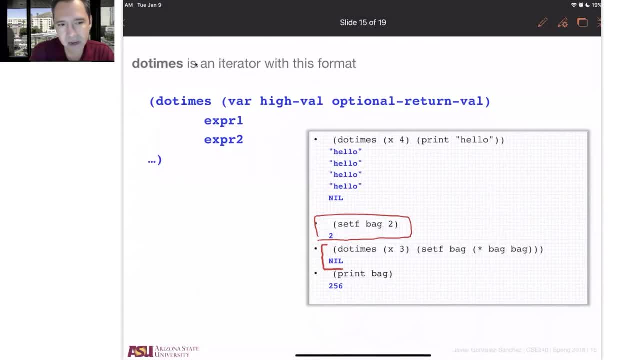 an example with more than one line. So line number one, open and closing parentheses. I have a new variable And that variable exists. from this point below, You create a variable, the variable exists And, in particular, this one is going to behave like a global variable. We're going to talk about global. 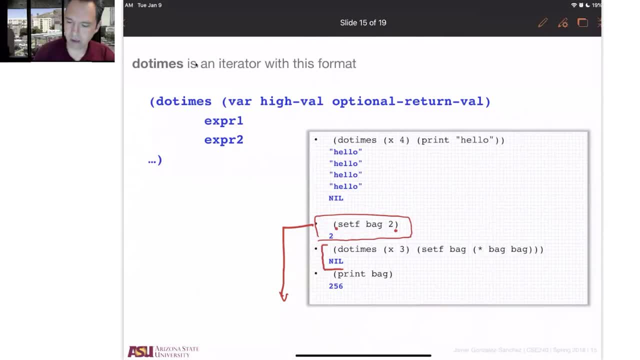 and local later. but this one is alone and you can think this one is global because basically you can use this variable, The one that you create with the set F, in any other line, So parentheses with the set F and any other thing that you put inside parentheses, doesn't matter how many lines. 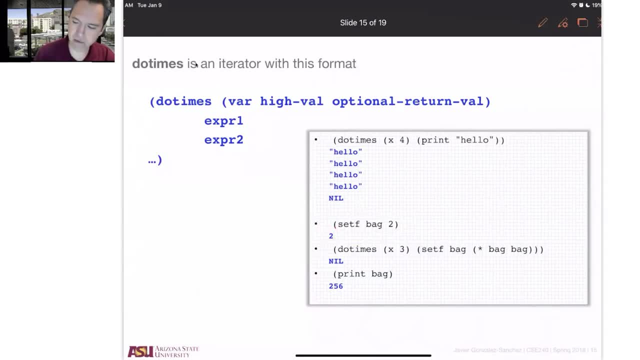 can use that variable from this point below. So two times, I want to create a for loop, The for loop, the variable that I'm going to be using, the name is X. How many times I want to run the loop? Three times What I want to do inside of the loop, this instance. 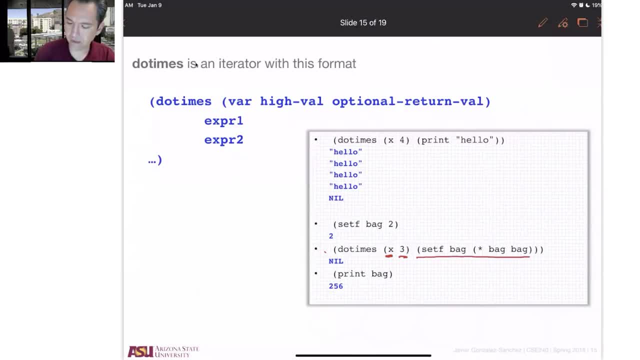 I'm going to do is I'm going to use the set F again. Yeah, Why? Because I need the equal. This one was like back equal to This is my equal And also create the variable. but because back do not exist. So, from this point below, back exists. 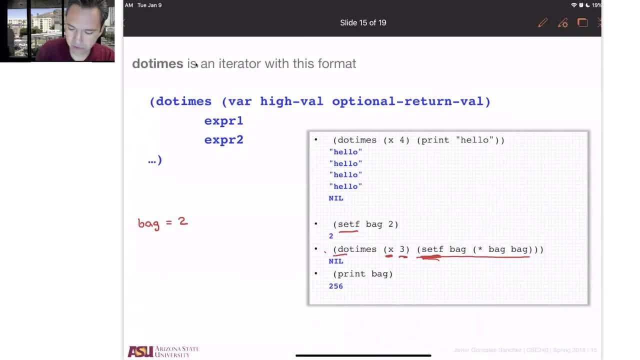 This line is a two times, Two times A for loop And I want to use the variable X- Okay, The variable X, And I want this loop to run three times. Okay, You want the loop to run three times. So usually Java CC++ is like: okay, we're going to start with zero And 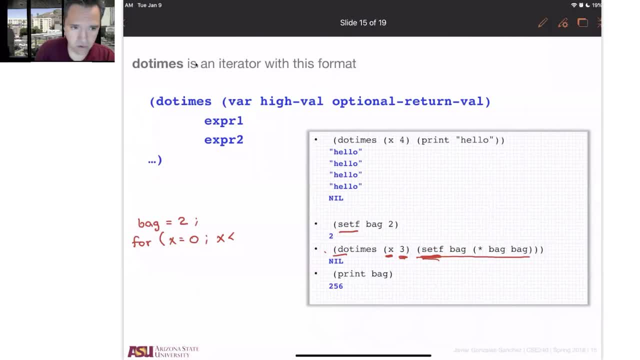 because you want to run this three times. I want to run zero, one and two And I need to increment the value of the variable. Now, the instruction inside, The instruction inside is okay. there is a multiplication And it's the first thing that is going to happen, because it's the inside parenthesis. 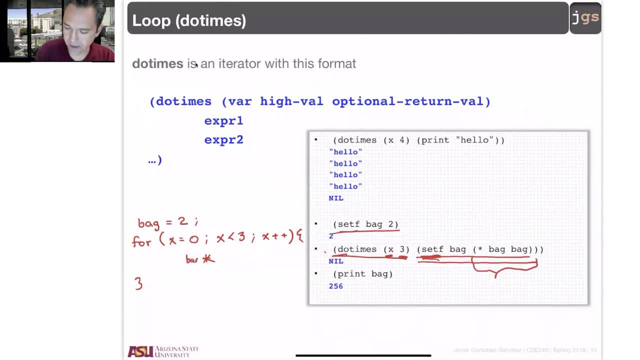 And it's a multiplication of back, Back, This part, And then that one is inside of this set F, And it's the second parameter. What is the first one? The same variable, And that is what I want to do. I have another instruction here. Notice, this one has another group of parentheses. 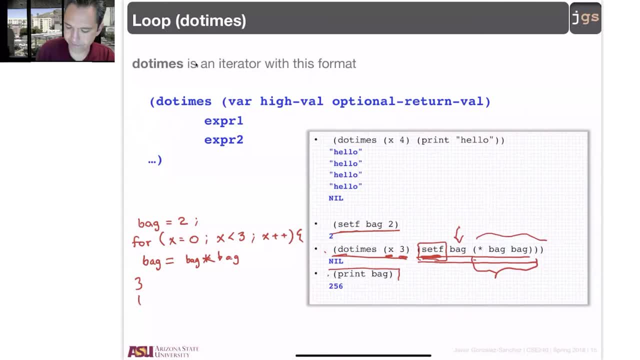 Print back. I want to print here, If I go with C, Something like this: So my programming list, The equivalent with C, And well, at the end, every single line is going to be printing for you the result. So set F. print as a result the two, because it's the value stored. 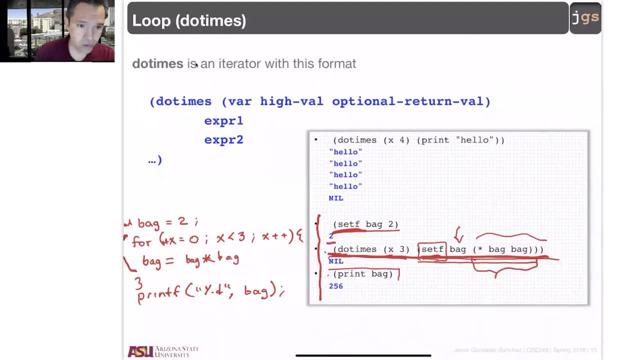 inside of the variable When you run the loop times, remember here should be the value that you want to return. If you put nothing there, the return is going to be nil And when you run print, it's going to be printing the value. And if you run the loop times, 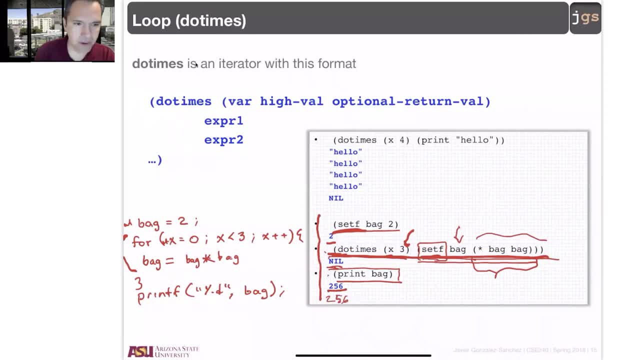 if you run this, you're going to notice the number printed two times One: the instruction print. The second one the return value of the function. Any question? Okay, guys, See you next week. Thank you.